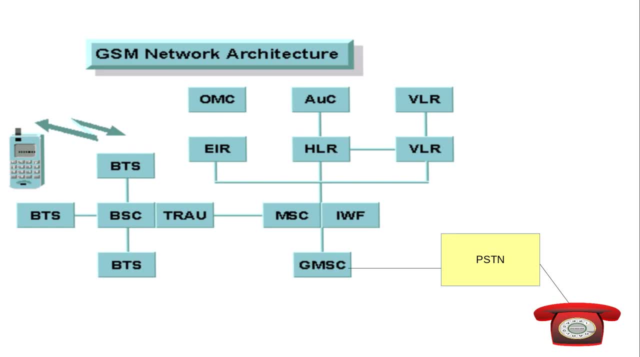 So how is this mobile station roaming number allocated Now? for example, this is the mobile station MSE, area number one, and it interfaces to the outside network using this gateway MSE And it is called the gateway MSE And it is connected to the PSTN network. 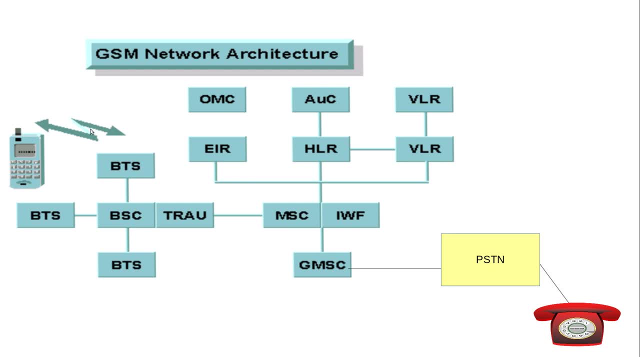 Now, if a mobile is in this MSE area, it is the VLR or the visitor location register, which is responsible for the temporary data, that would allocate the mobile station roaming number to this mobile, And a copy of this mobile station roaming number would also be in the HLR. 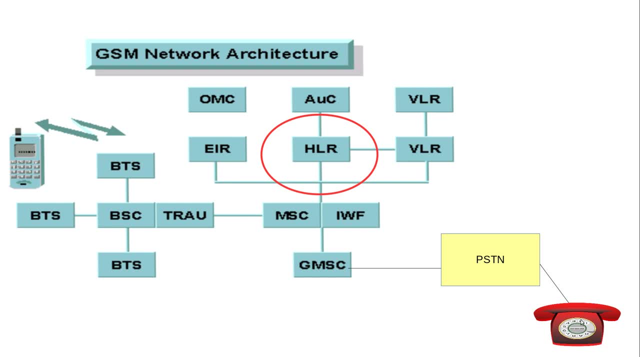